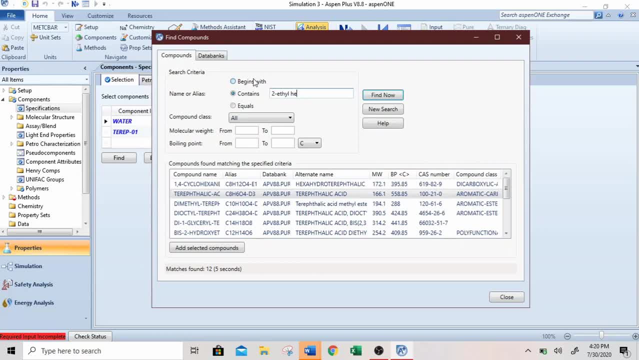 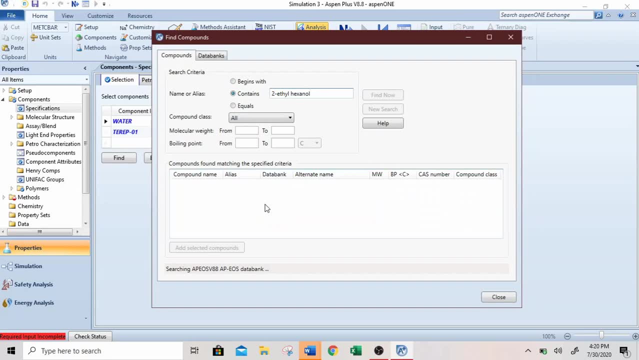 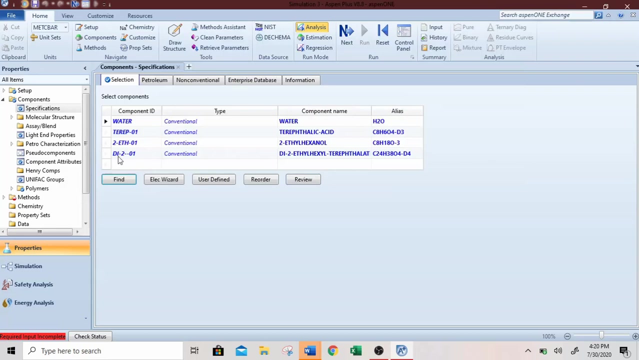 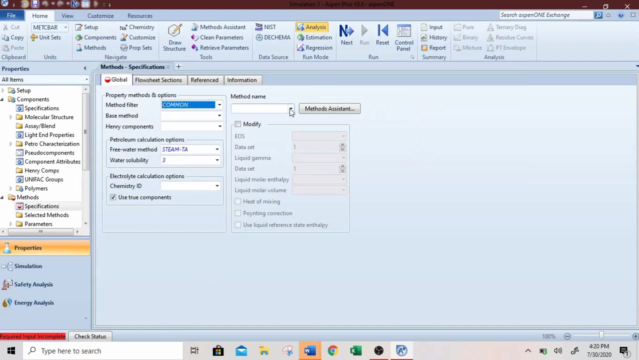 two ethyl hexanol. it is basically a complete name: two ethyl hexanol. don't mess up. you see, we directly find out now. only we have di octyl tethylate, our main product. okay, so we will click on the next button. we have to select method. any one of you who 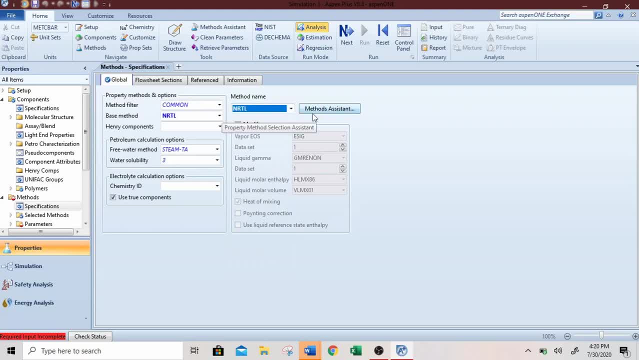 previously used. any simulation software of chemical engineering is probably aware of these methods. you need to use accurate, appropriate method for your system. it varies from the reaction system, from one reaction system to another reaction system. basically, you can study your matters in method system or you can use Google to select perfect matter for your system. you basically need 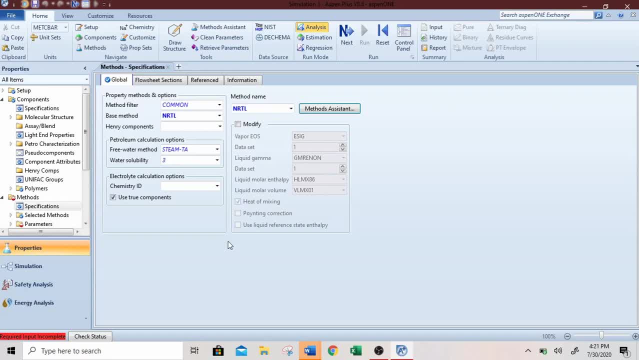 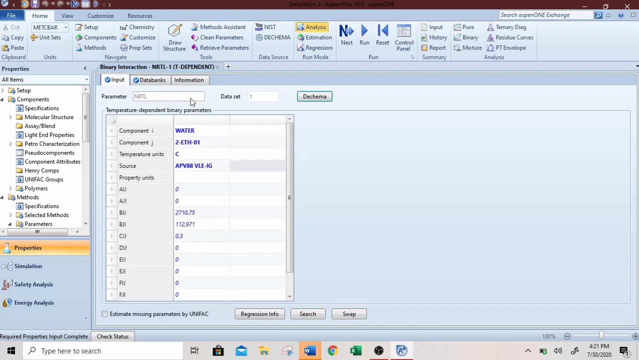 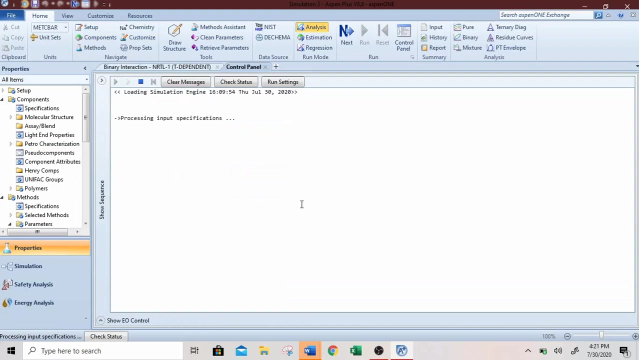 be avaialble data and thermodynamic equation. or you just create the data in the matter, or you aj q cirvate your model gamma, xn李, meta and Google. i will make separate video on this topic: how to select and appropriate models for your system. however, with google newton, the others are uh, things like that. will make separate video on this topic: how to select an appropriate method for your system. now we will click next. i do eventually click this next again. click next than property nulls is okay. now it will be carrying processing input specifications to generate activation data. output in information with data. whatever the databases all located after data we have to create ощущated expoutez our data and use these to generate atmosphere data. ouräs avechata y today we will make a separate video this way. Tikdu folks. ok, the尤 ahen operation model is perfect, so if it gets them a separate video this way, but they are very sensitive because anyway, 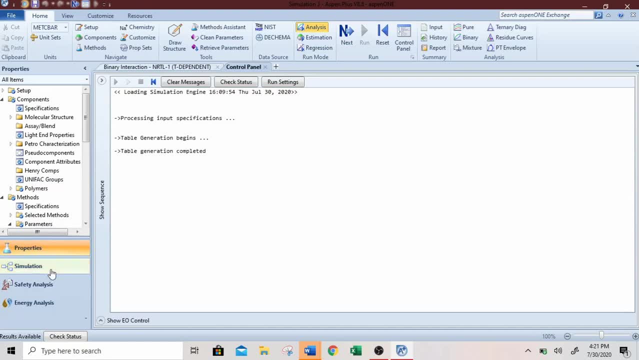 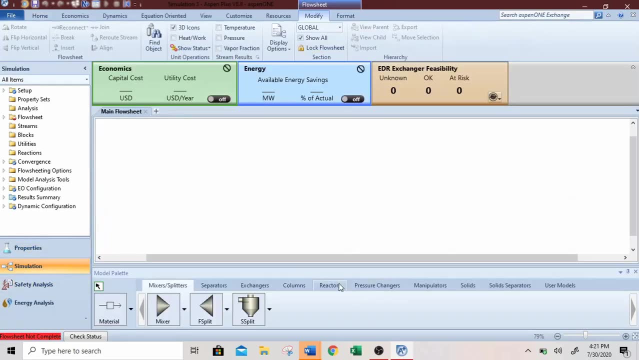 we have to create scholarship and then another proci super cyber, cyber, levelujemy the data internally and etc. will be courageous it needs for your system. now we will move it into our simulation system. we are basically designing a simulating a batch reactor, so we will add our odd. 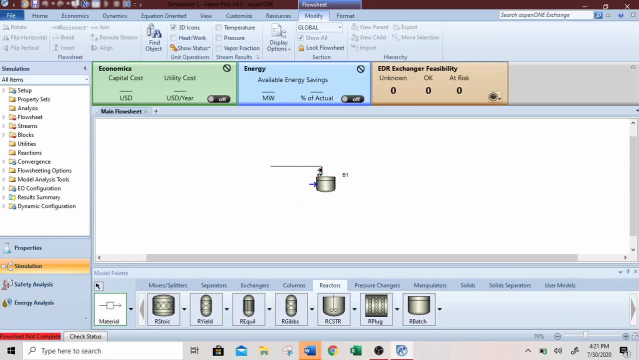 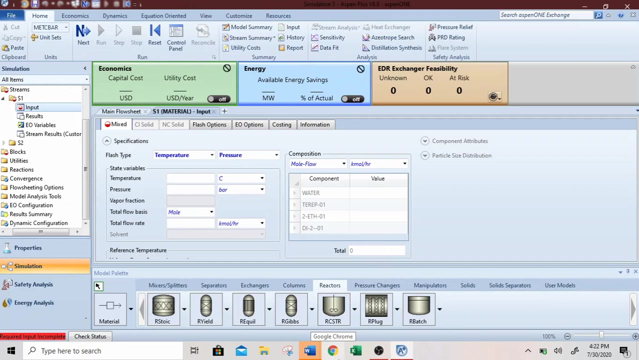 batch, we will add our input steam. the red one is our process team and blue one is our utility team. we are not using their precise data by putting utility steam or something, something else, we are just putting in the processing. now some of you might be thinking we have, we are using a batch reaction, batch reactor. 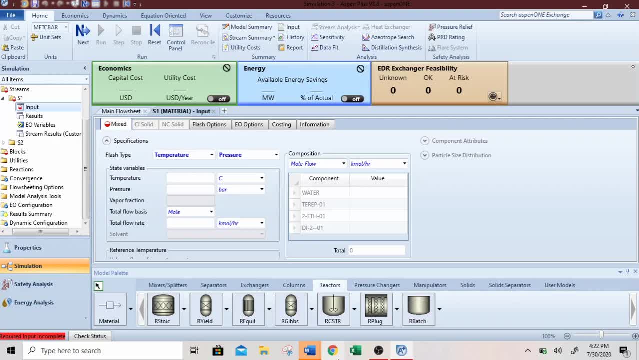 basically why we are putting in the input stream. I think as far as I know about this Aspen plus, there is no way to add a batch steam or batch directly without putting in continuous stream. so we will use our mass basis in by putting all the mess in per hour form, and I mean all the 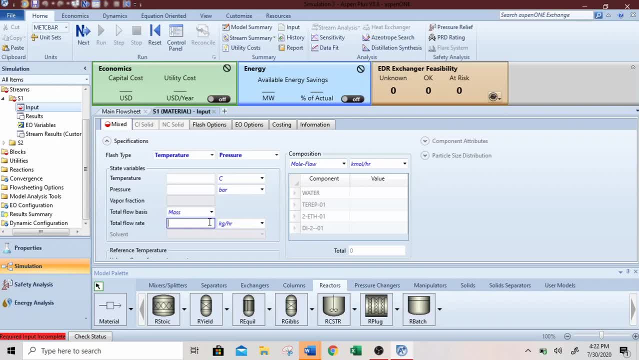 all the batch in kg per hour form. for example, I have 19,000 kg batch. I will put 19,000 kg per hour, neglecting the per hour addition. we had a reaction temperature of 220 degrees. you can verify your case as, as you are already probably aware of it, we have a reaction taking place at atmospheric 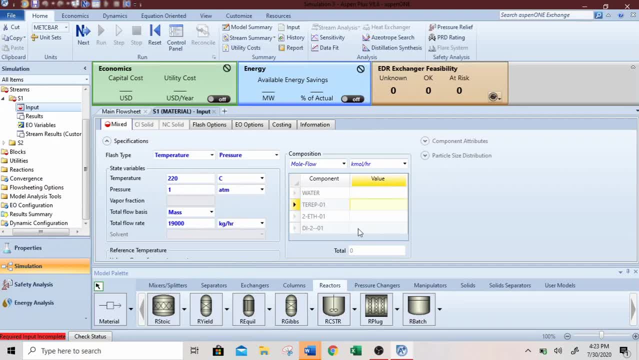 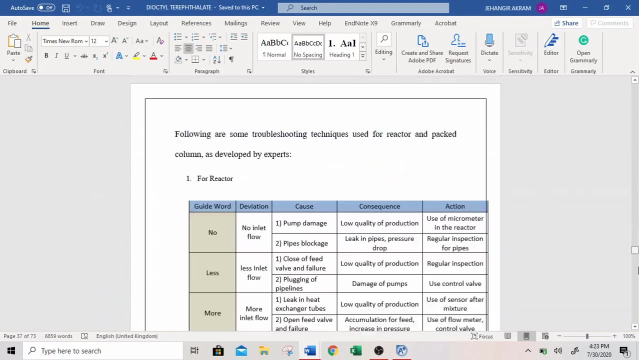 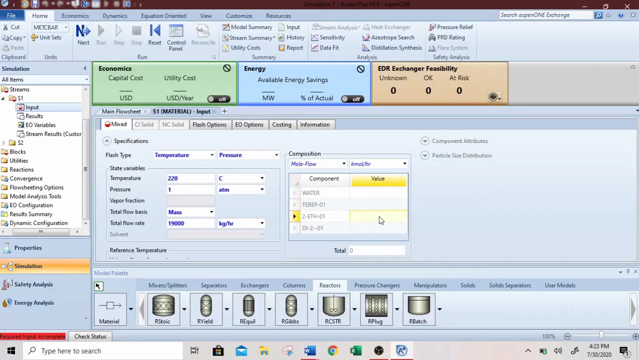 conditions. now we don't have butter and diacrylate in our input into that, but we have. we do have alcohol and tartaric acid. okay, i probably have this information already. i carried out this simulation earlier- 0.63. you will get this information from your material balance. 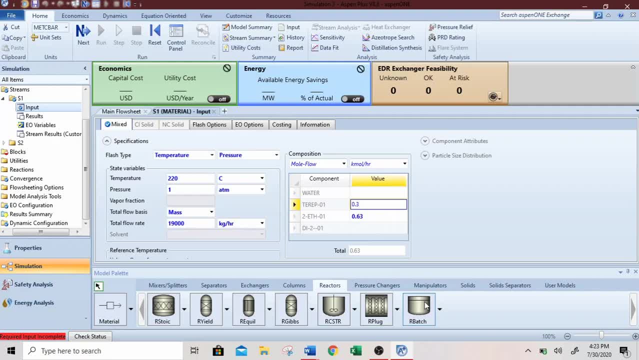 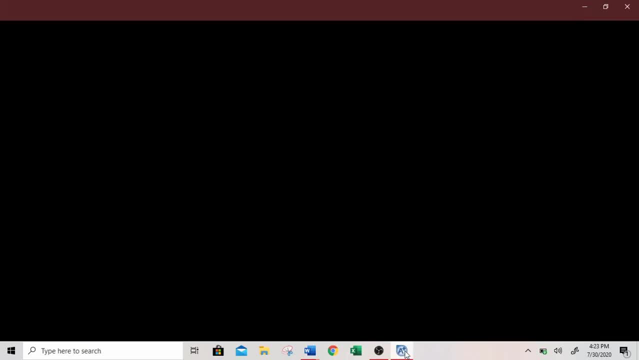 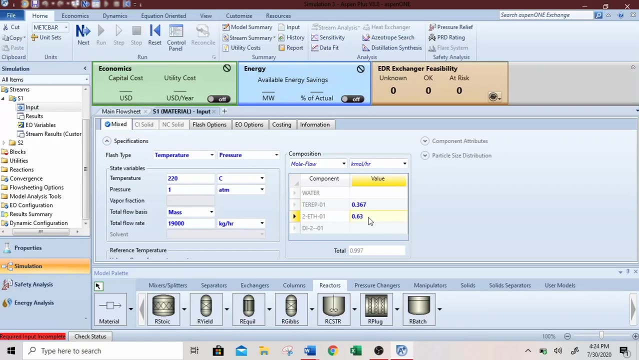 i think i don't have to remind it again and again you you need your material balance before you can design, assimilate your reactor in. i am basically using 10 extra alcohol, which was recommended by the patent owner, to get efficient, high efficiency of reaction conversion. now we are in the reactor, which is the main. 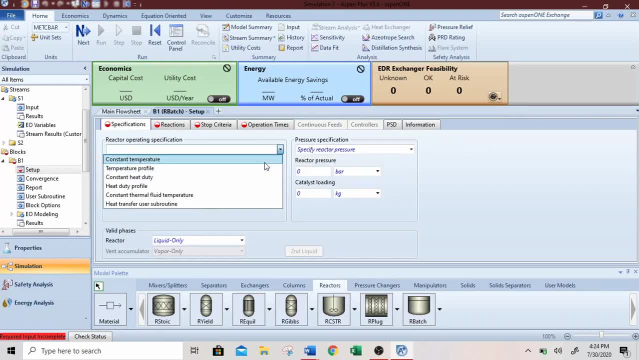 specification area. we will be simulating our reactor as a constant temperature vessel, constant temperature reactor taking place at 220 degrees centigrade taking reaction and one atm pressure cataleas. loading in our case is 33 kg. you will get all this information from here. 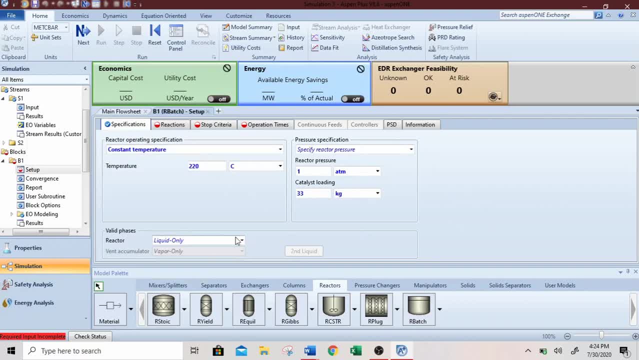 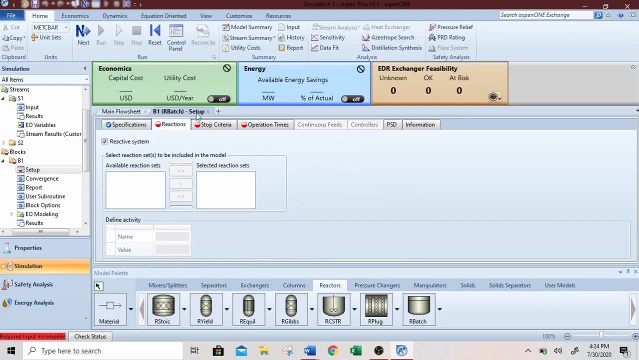 from your reaction kinetics data, which in my case, is already specified. I use Google and various research papers to get this data. you know that you need first order, second order reaction kinetics data. you study various regression models to calculate these values. now we are in the reaction section. most of I 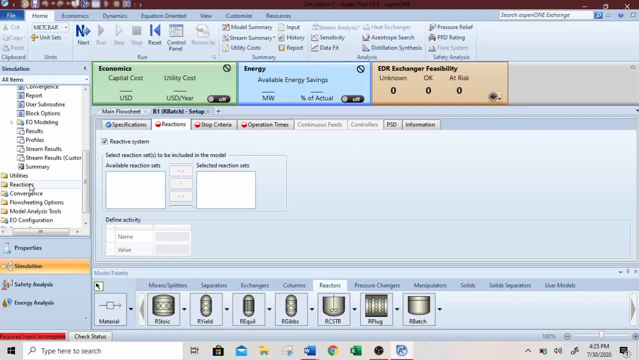 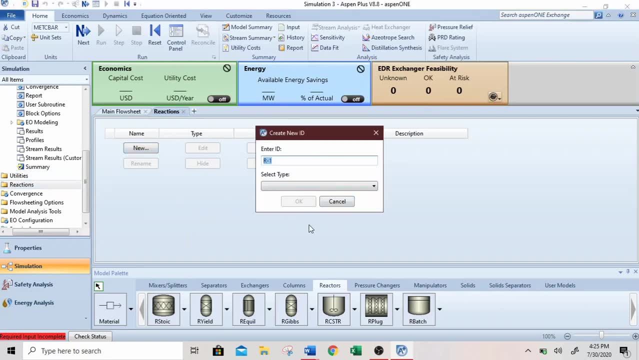 most of us are, and including me. I got confused in this portion- how to design a reaction or how to insert a reaction in Aspen plus. so I use various sources and books and videos to learn how to create your own custom reaction in Aspen plus. it is not so difficult. basically, I call the reaction as R1. 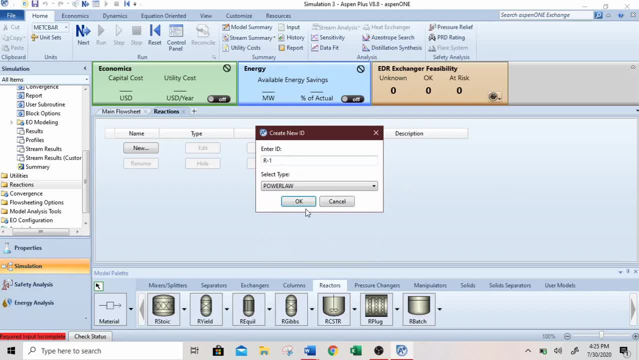 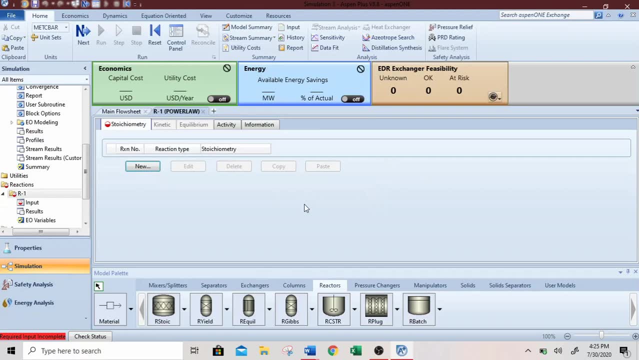 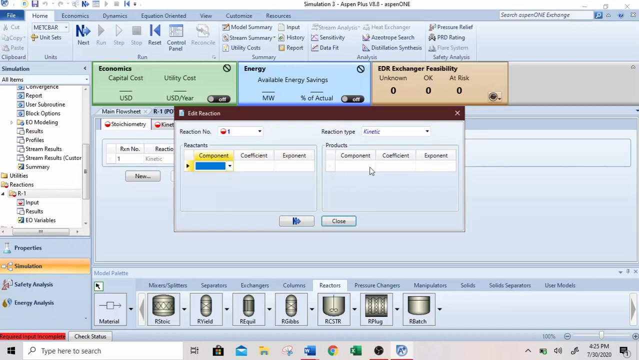 now I will select power law model, power law type to specify my reaction reaction. I don't know how do you other model? I basically will use power lock in my case. maybe you know better matter, better models for reactions, then I do so you can try other model. basically, this is reactant section. this is product section. 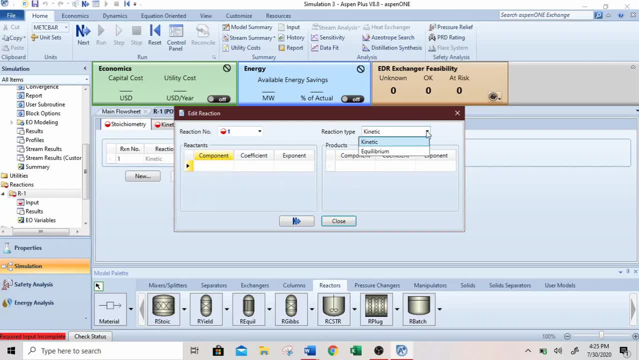 I am simulating my reaction as kinetic, not an equilibrium reaction. that's a late, rapid tweet. I'll have you know to make. what is the direct and water? we are simulating it as. with respect to product. okay, ready question. with respect to products, yeah, it means that we have minus one. 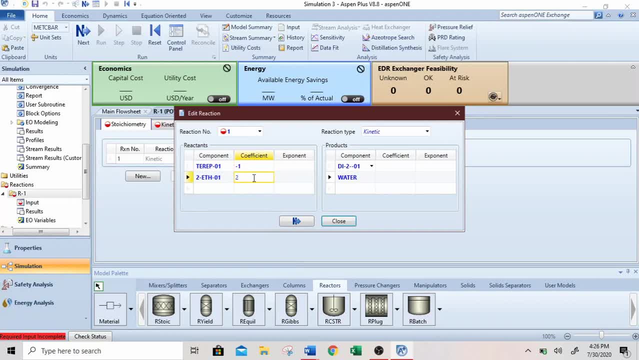 okay, ready question. with respect to product, yeah, it means that we have minus one, minus two, one, one exponent, its coefficient is one, its coefficient is two. one will, of the late, react with two motor to tell you not to make. one mole of do TP and two mold of water exponent in case of products is zero, zero and in case of 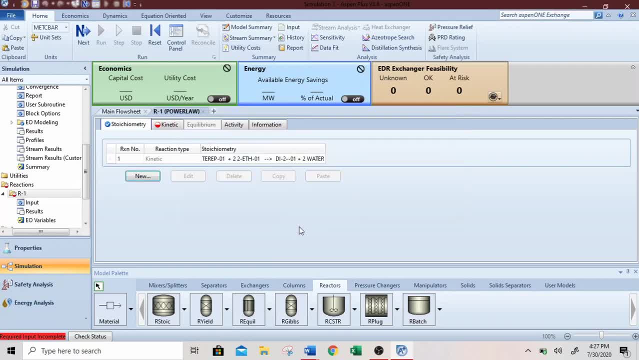 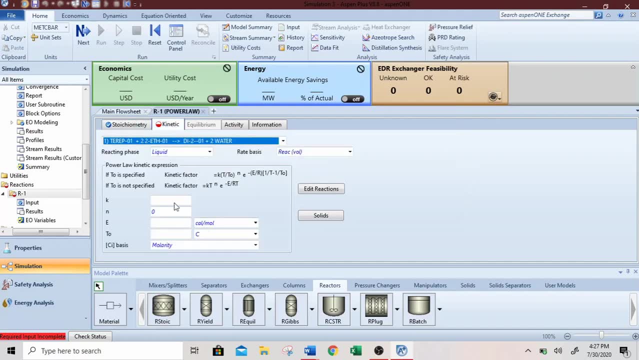 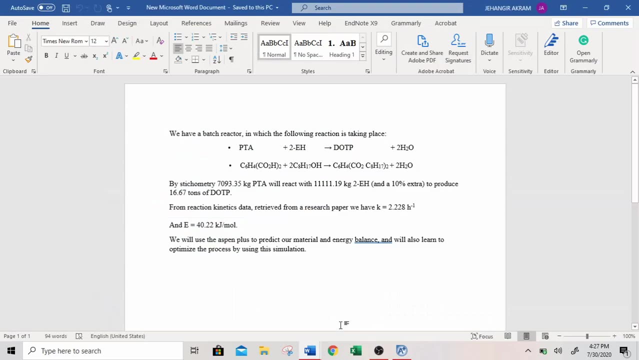 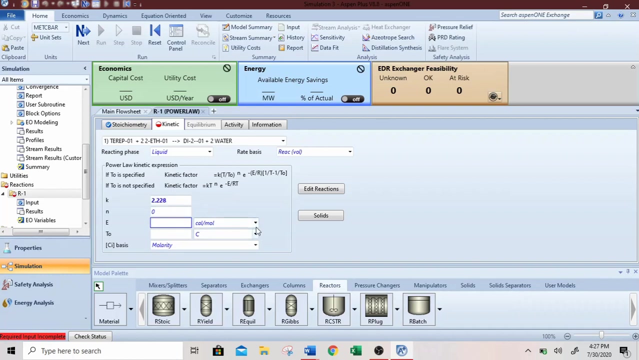 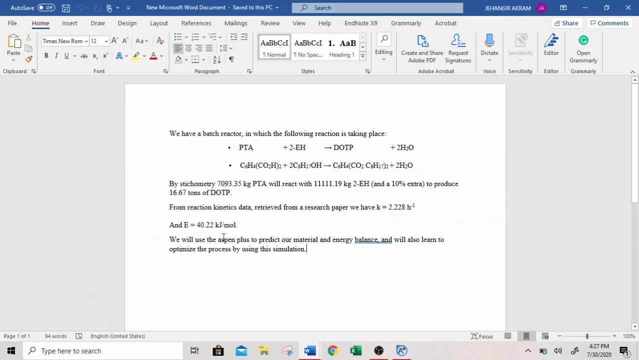 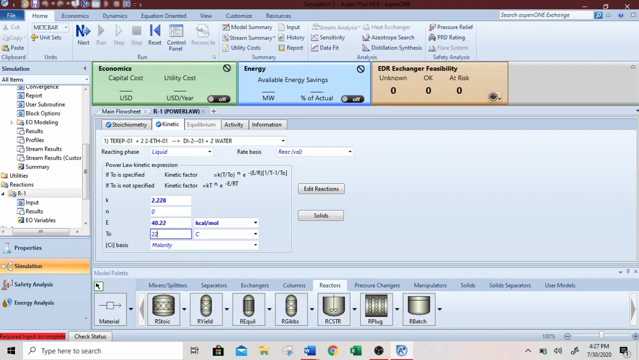 you can only measure by making a meter of the reaction. is one K between. into some information we need to enter the value of K, which in our case, in our case is 2 V of kilojoule, 40.22 kilojoule per mole. you can specify it at 220 degree centigrade V. 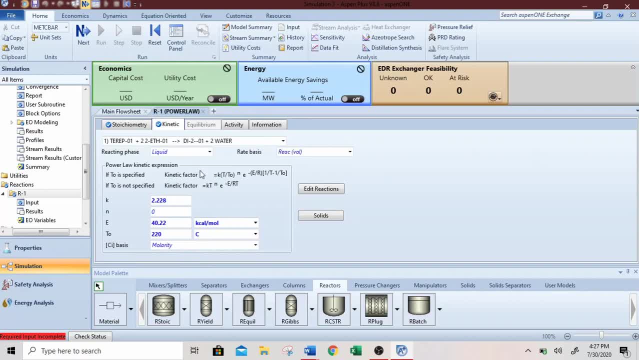 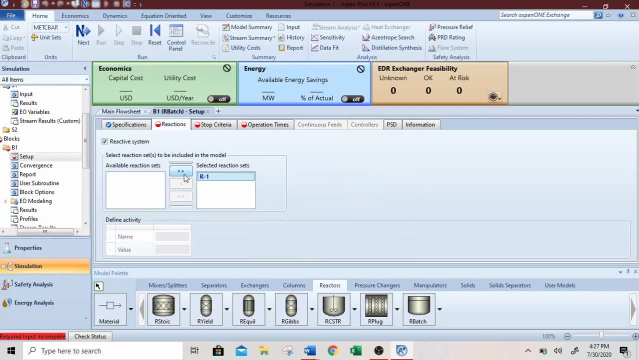 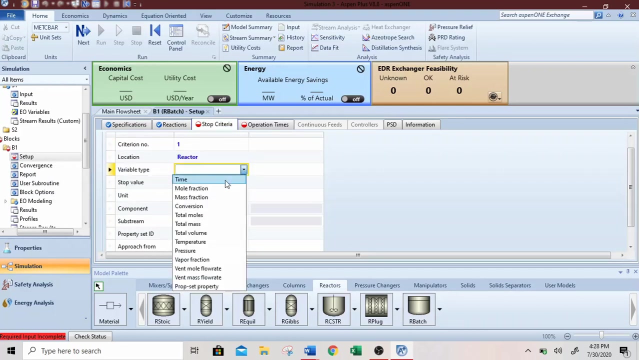 and leave the n as 0. now click on next button. ok, now we are in the reactor again. double click on the reaction or simply arrow button. now you can. you can select your own stop stopping criteria for react batch reactor, but I will specify time as a variable, for as a mean of 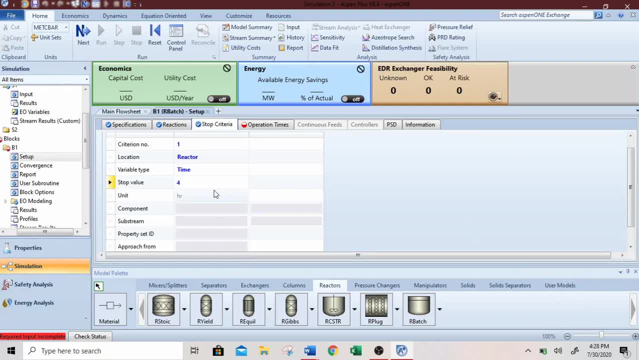 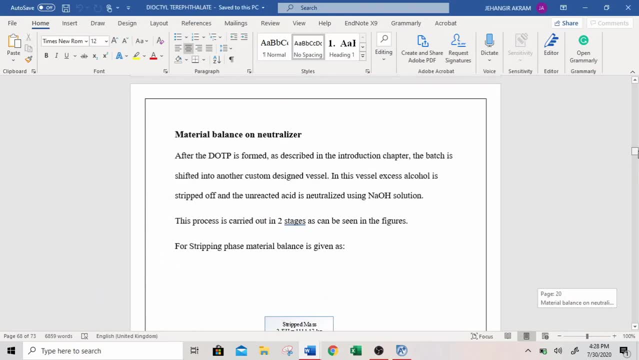 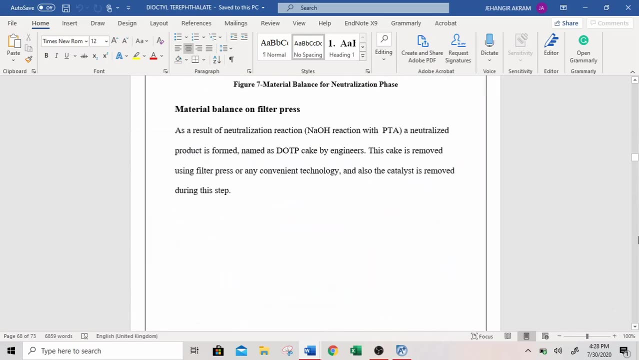 stopping the reaction. stop value: 4 hours. basically, I will allow it to react for 4 hours, which I already calculated myself. it is not based just on the assumption. I have already calculated it. The appropriate value is around. I will show you where did I calculate. see from first order. 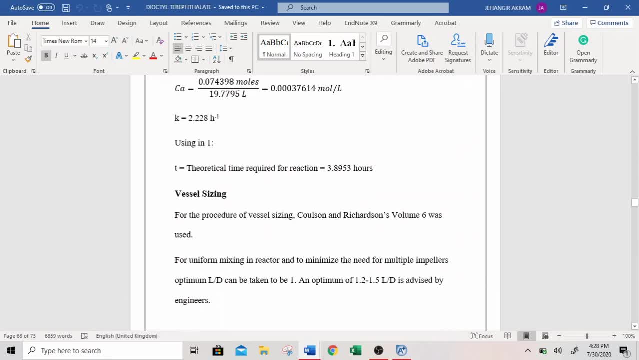 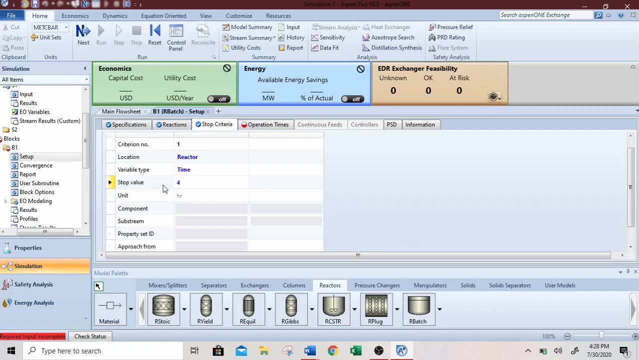 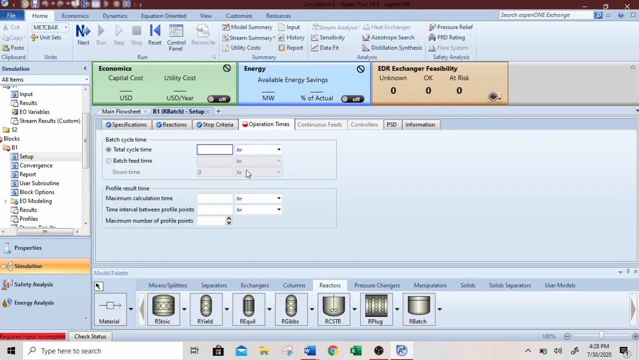 react rate equation. I calculated the theoretical time required for the reaction to be almost 4 hours. 3.89. almost 4 hours. ok, which I? it is already specified, no need to specify anything else. Now I will calculate the baseline total cycles time. you can see its descriptions for all. 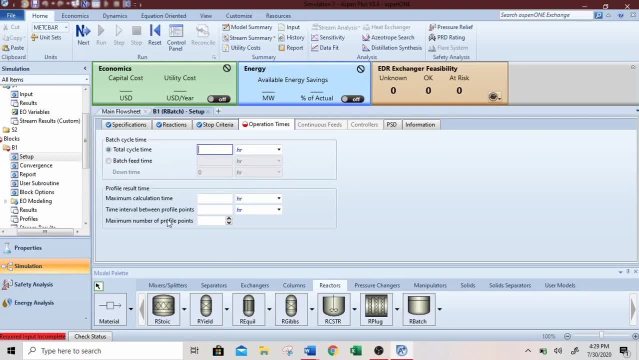 the fields must be entered. reactor cycle time. what if we specify batch total cycle time? you can call it as 4 hours. ok, now maximum calculation time: 2 hours time interval between profile points and no, no, no, no. maximum number of points. leave it to be 3, okay. 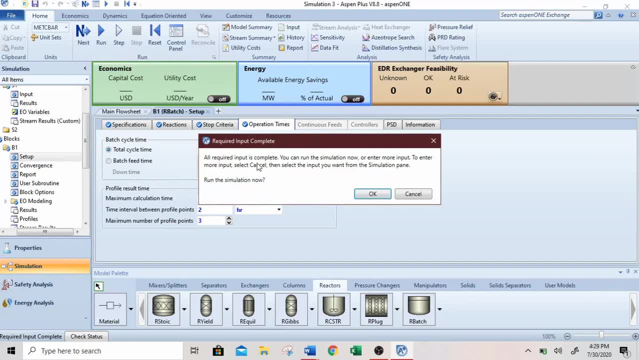 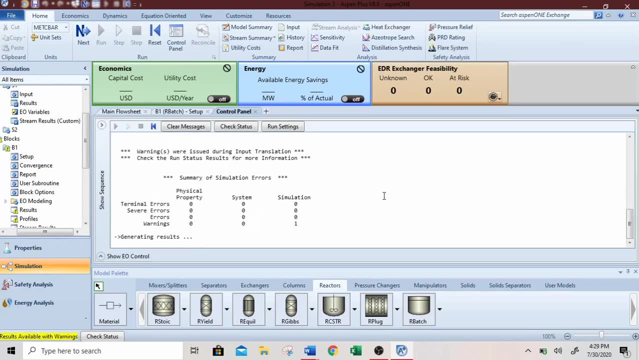 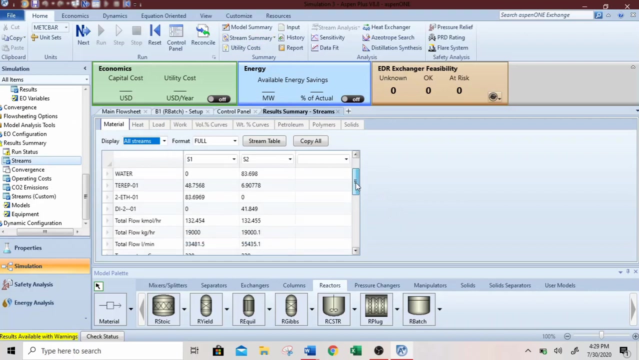 now click Next. it is saying all the required input is already complete, so we will run the simulation by pressing ok. it works available with warnings. warnings during. let us see our steam summary to see what are the warnings: oh yes, oh yeah, I think our modeling is almost complete. you see that forty one point.